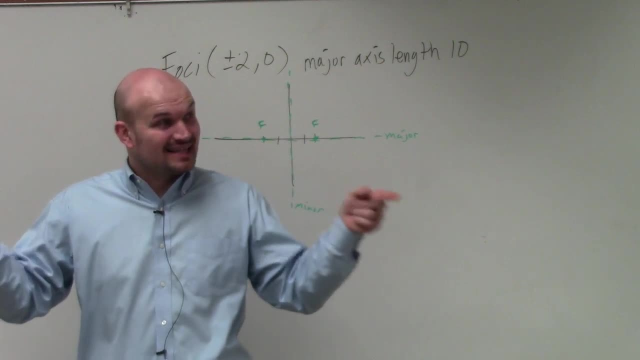 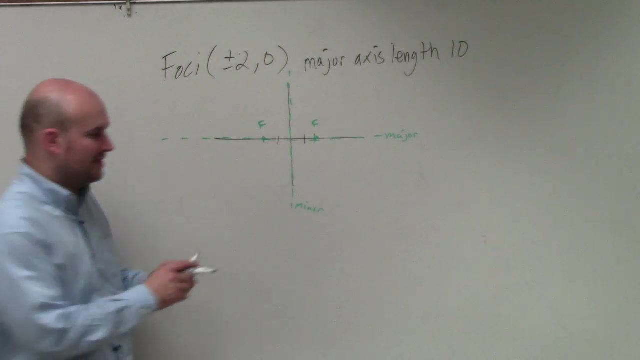 Well, that's separate. So you can see that the center is exactly in the middle between your 2 foci, Right. So I look at my 2 foci, I see the distance between them is 4.. So, therefore, the center point is going to be at 0, 0. 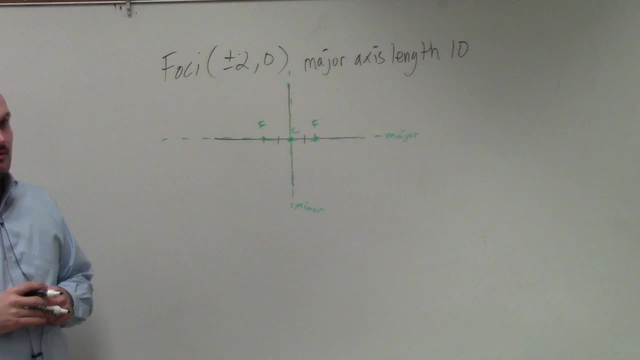 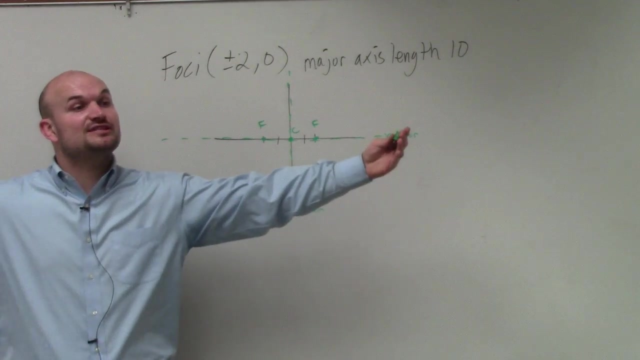 So I'll just do center, Follow me. No, The center is in between the 2 foci. Here's your 2 foci. Center is right in between Right. So 10 is from one vertices to the other vertices. 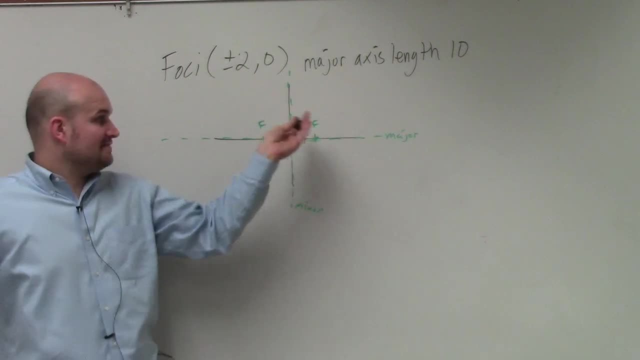 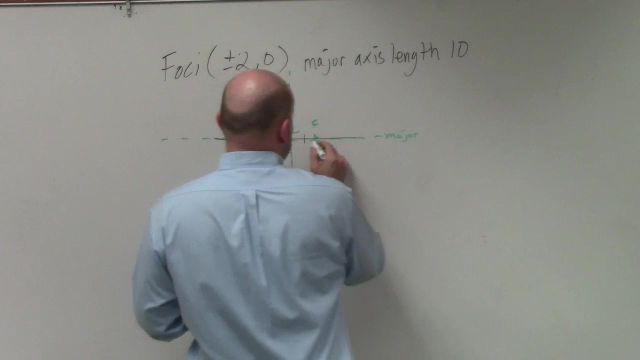 Right. So from vertices to vertices. No, not the f, That distance is c, That's 5 on each side, Right? So let's go and do that: 1,, 2,, 3,, 4,, 5.. 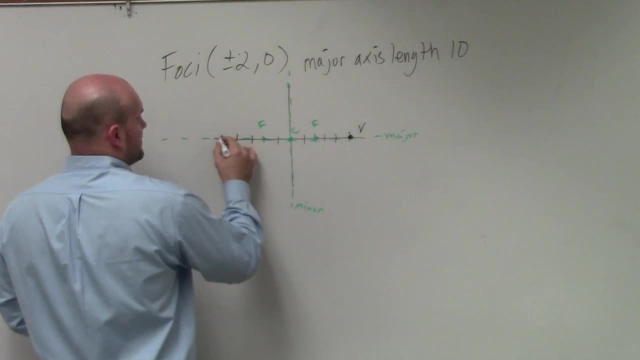 Vertices number 1.. 1,, 2,, 3,, 4, 5.. Vertices number 2.. Right, Okay, We're doing pretty good Now. So we know that this value- the distance from the center to the foci- is c. 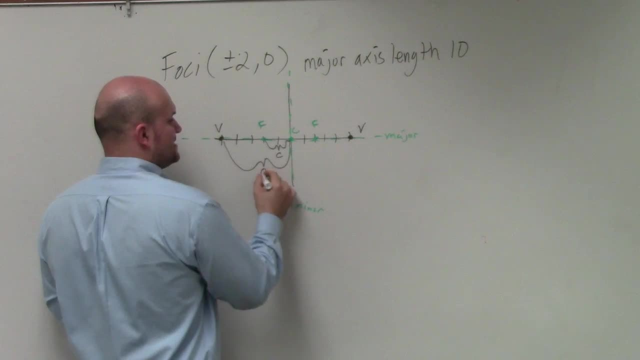 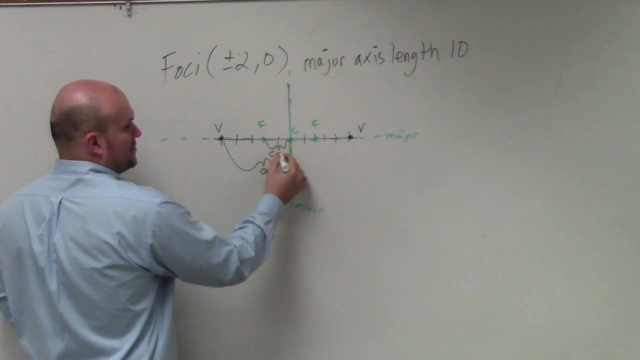 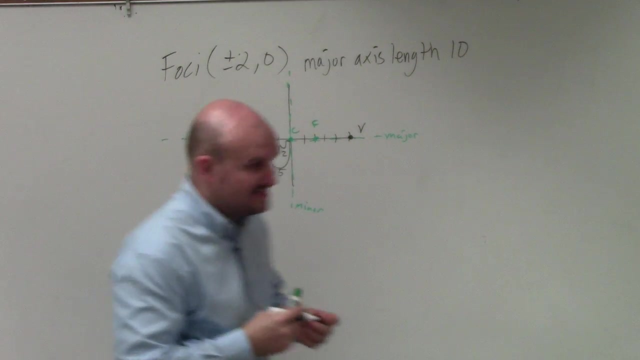 Whereas the distance to the center, to the vertice, is a Correct. So we can just look at our formula here and see that c is equal to 2 and a is equal to 5.. Does that make sense? Now, c is not a part of our equation. 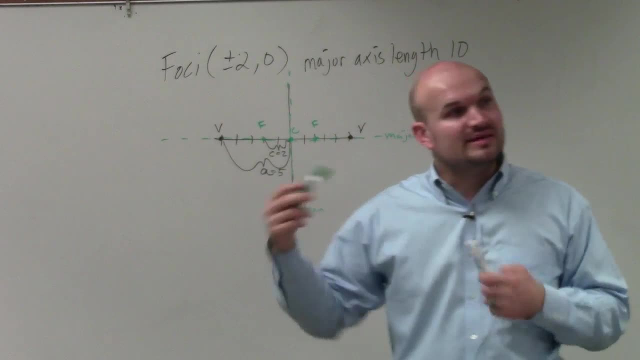 If you guys look at the equation, c is not a part of the equation, Right Right, But we did talk about c. It was actually written up there and I actually do a part of it. I didn't write it down. 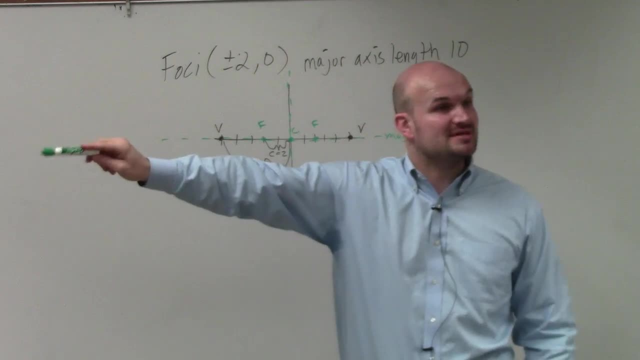 But if you had your book, you could have seen the equation for c, And we also did problems like that, So you guys should have had it written down on your notes, anyways. Right, All right, But before I even get to that, 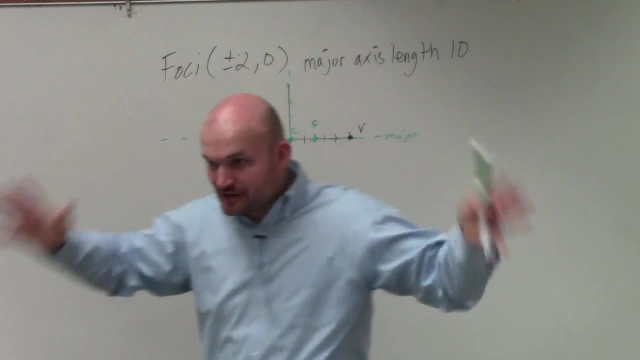 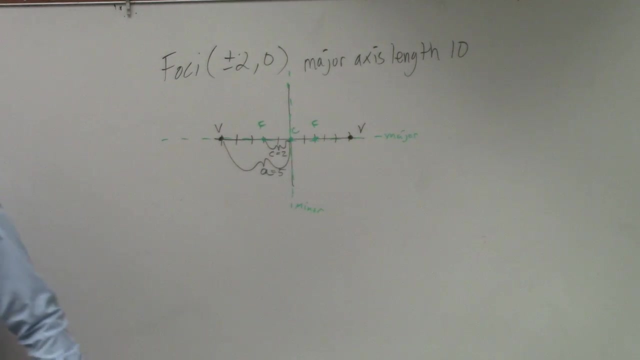 The next, the most important thing. So now I've plotted the information, All the information I've figured out. So that's step 1.. Step number 2 is to decide which equation we're going to use. This equation is when you have a major axis that's horizontal. 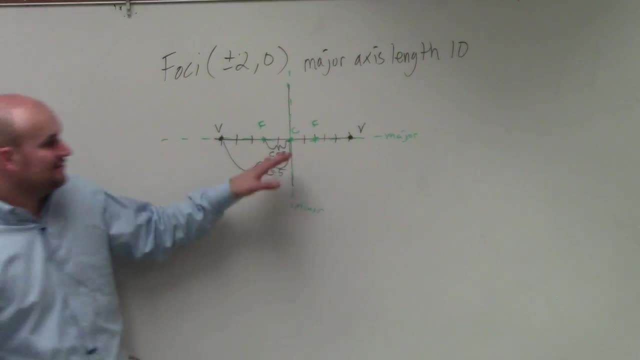 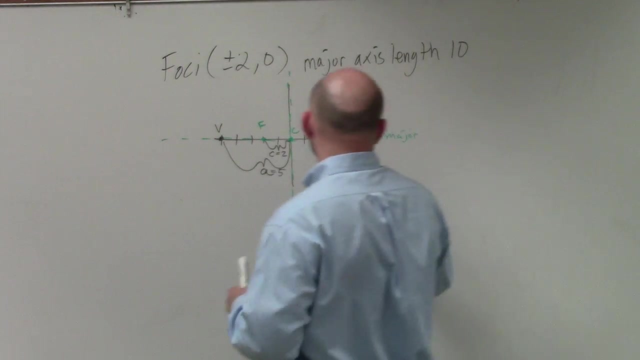 This equation is when you have a major axis that's vertical. So therefore, since my center, my foci and my vertices all lie on this major axis that's horizontal, I know my equation that I'm going to use is going to look like this. 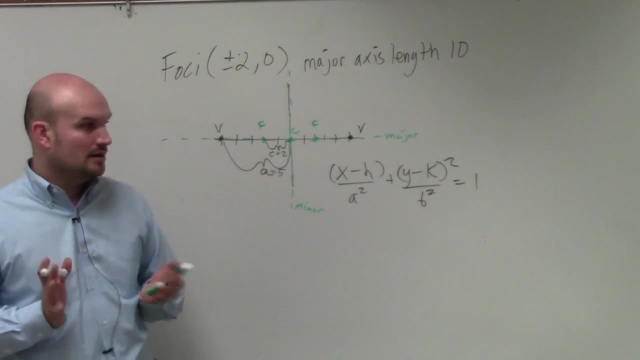 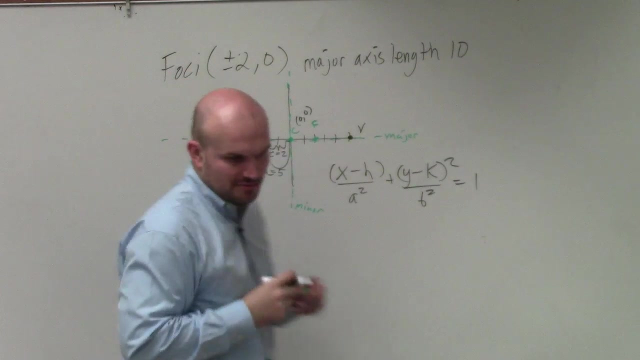 Does everybody agree with me? Yes, Okay, So we have our center, which is 0, 0.. So we know that is going to be: Bless you, Bless you. Somebody stole my red. There we go. So we know that my center is H and K. 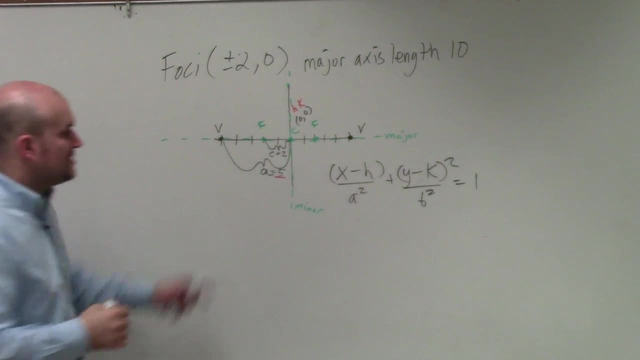 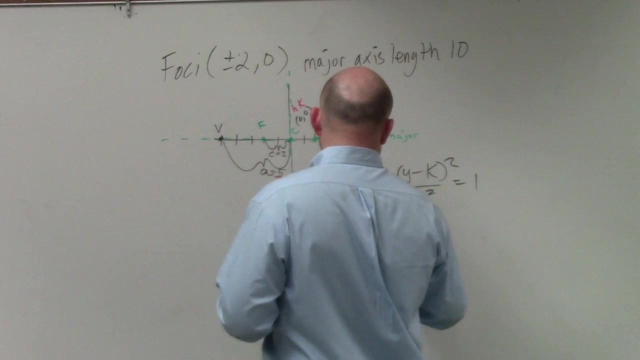 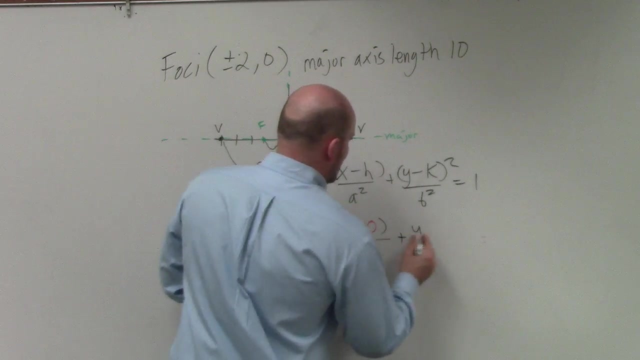 We know C is 2 and A is 5. So I can plug in that. So let's plug in the information we know real quick. So we have X minus 0, which is your H all over 5 squared plus Y. 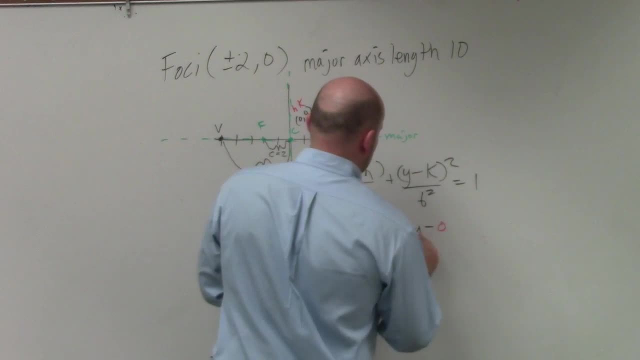 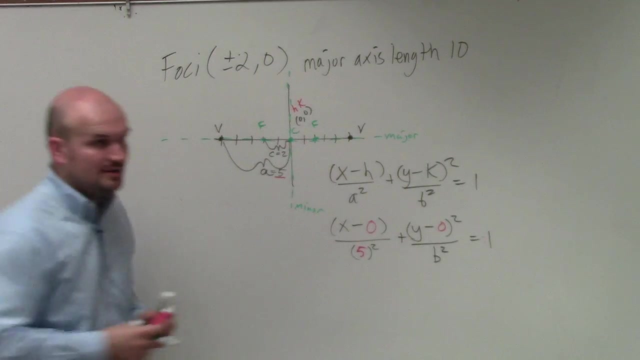 So we have Y minus 0 squared over B squared, But we don't know B squared, do we Right? We don't know B squared. If you guys remember, on Desmos, and what we worked on is, we have this formula that helps us talk about the relationship between C squared equals: 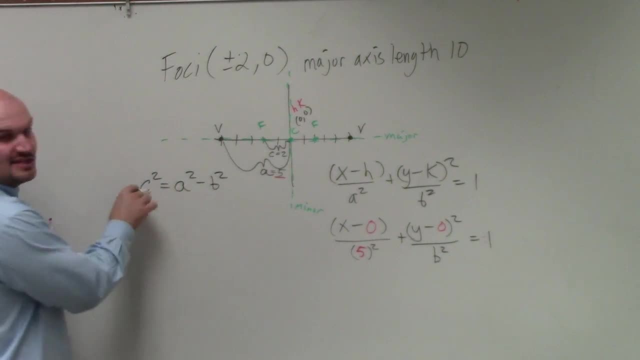 Well, it's C squared, A squared minus B squared, and then the solve for C. So if you want to solve for C, you can, You can go ahead and plug that in, Or yeah, I mean, you could easily just rewrite it like that. 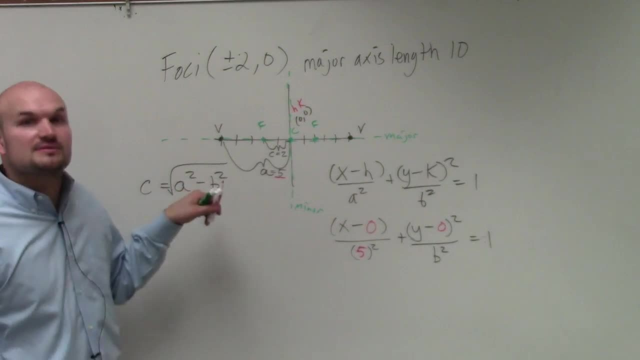 Right, Isn't that how we learned it last? Yeah, that's how it was written on Desmos: Good job, All right Now. so it doesn't matter. if you guys want to, Let's just you know, let's write it like this: 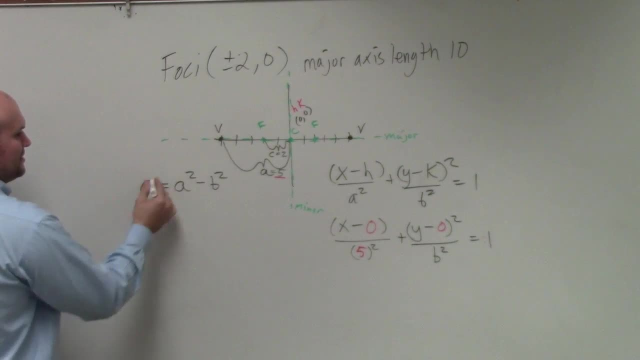 So we know C is equal to. Actually I like to use the squared one, So now I'm just going to plug in: 2 for C Equals 5 and for A minus B squared. So this is: 4 equal to 25 minus B squared. minus 25 minus 25. negative 21 equals negative B squared. 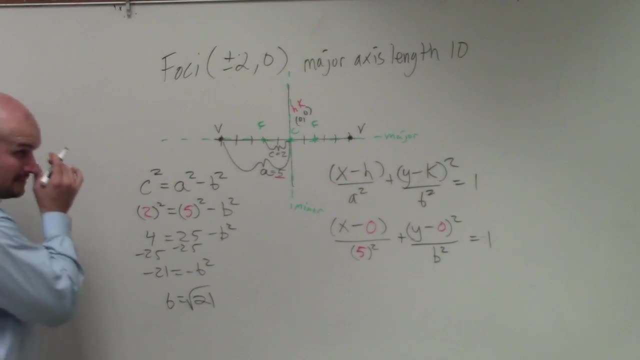 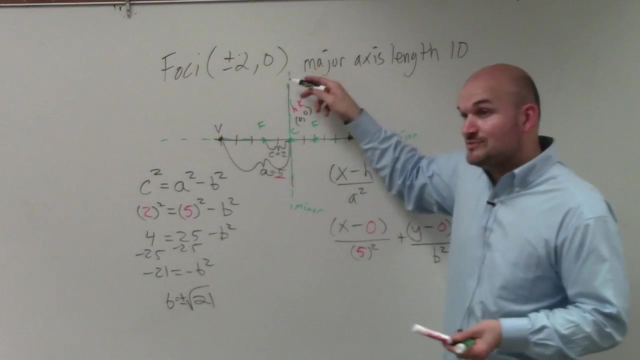 B equals the square root of 21.. In reality- sorry that- equals plus or minus the square root of 21.. Right, Because, remember B, you go up, up, square root of 21, and down, square root of 21. Right. 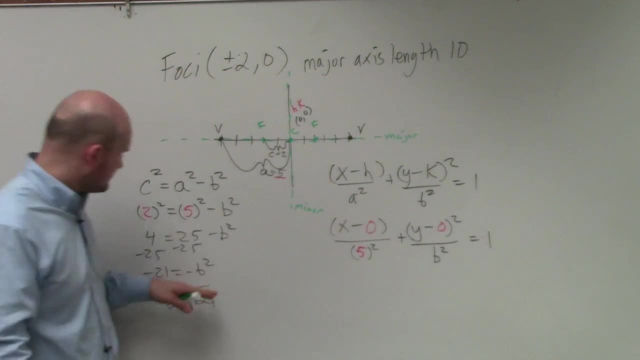 Now also. So another thing just to remember: isn't isn't actually you don't even need to solve for B squared? I don't know why, why I solved for B, But one thing: The square root of 21 always has to be smaller than 5..